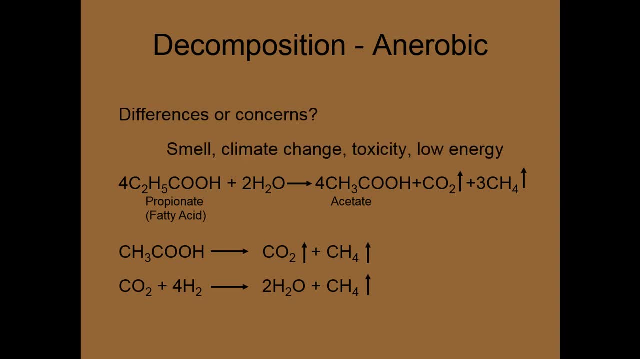 Anaerobic decomposition yields. biggest difference in its yields are the methane, the CH4, which is smelly and a much more effective greenhouse gas, So it can increase climate change effectively. Aerobic decomposition can cause toxicity and provides much lower energy outputs than aerobic decomposition. 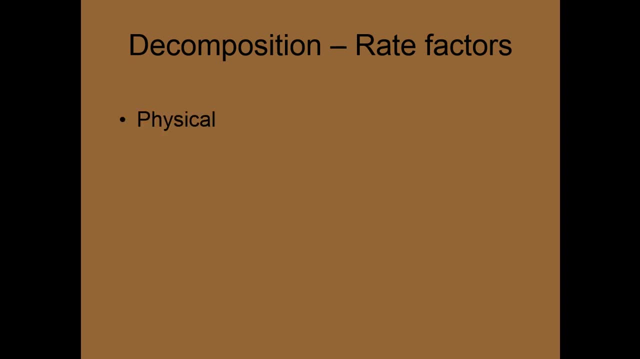 Factors on the rate of decomposition are physical factors: the carbon to nitrogen ratio, nitrogen availability around the material, soil, ecology and the lignin content. These are some of our Top five rate factors. So, physically, location in the soil profile, right on the soil surface, you know conditions are highly variable. so if we move down a little bit, have it incorporated into that A horizon, we have a much more consistent. 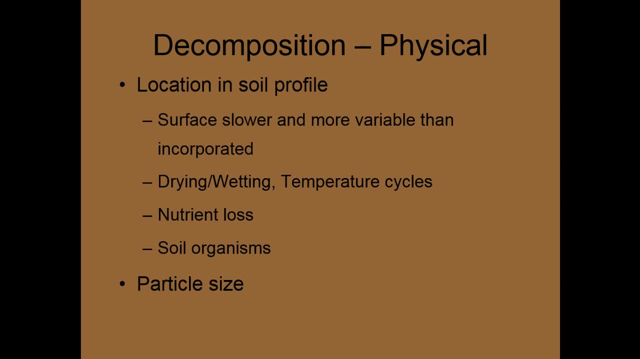 contact with soil, microbes, consistent soil moisture and aeration, things like that. Drying-wetting cycles, temperature cycles, all have an influence and then the soil organisms present. Then we have particle size. So if we think of a large branch falling on the surface, 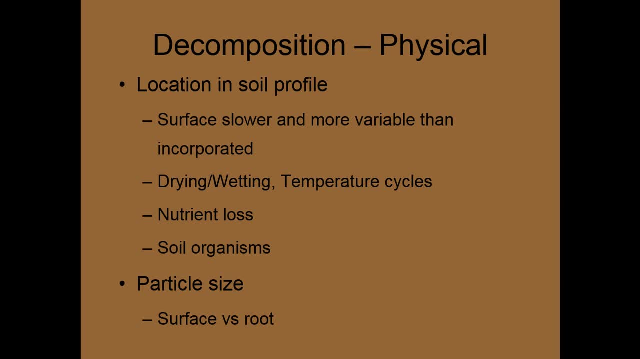 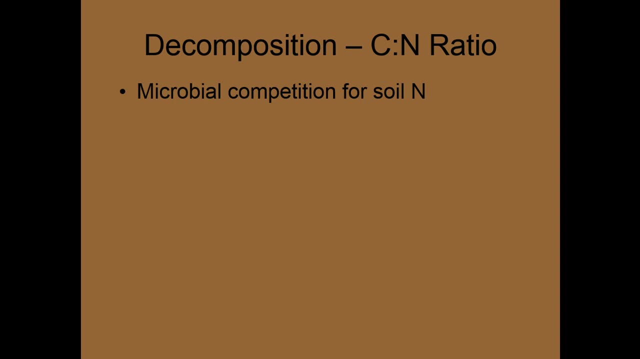 versus a fine root being decomposed and turned over Carbon to nitrogen ratio, So microbial competition for soil nitrogen. Plant carbon to nitrogen ratio can affect the decay rate and is variable based on nitrogen availability. So green legumes have about 8 to 30 carbon per 1 nitrogen. 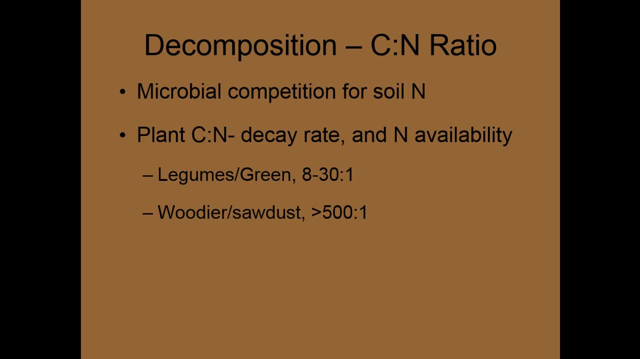 Something like sawdust can have as much as 500 carbon to 1 nitrogen. Microbes are a lot less variable, So they're usually 5 to 10 carbon for every 1 nitrogen, And decay slowly decreases this ratio, So the more extreme it is, the longer it will take to decay. 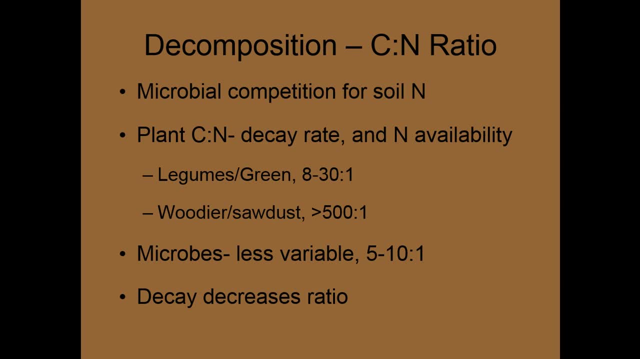 You know, if you think of putting a pile of sawdust or chainsaw material on the soil versus a pile of fresh soybean material, the soybeans will decompose and be unrecognizable much faster than that sawdust would be. 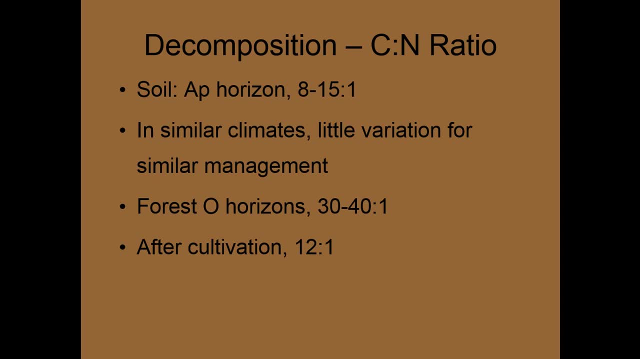 In the soil. a typical AP horizon has a carbon to nitrogen ratio of 8 to 15 carbon for every 1 nitrogen. Similar climates: there's little variation based on management. Forest horizons can be up to 30 to 40 once cultivated. 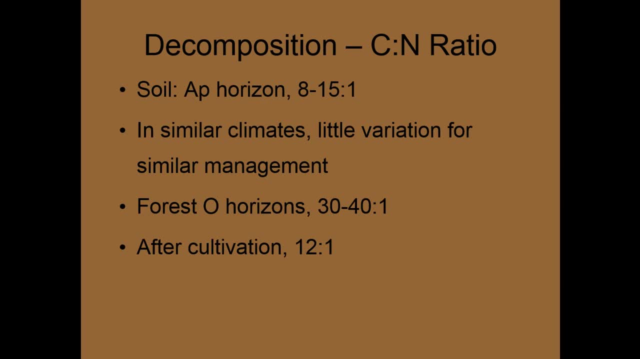 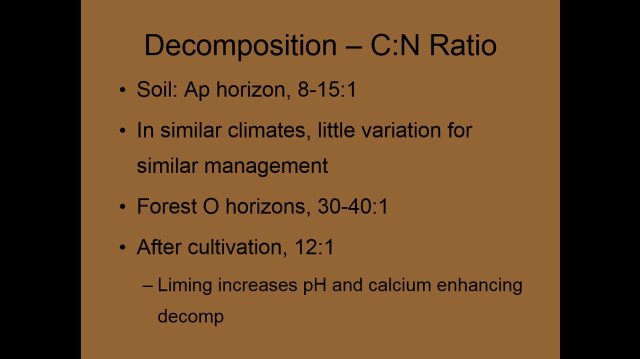 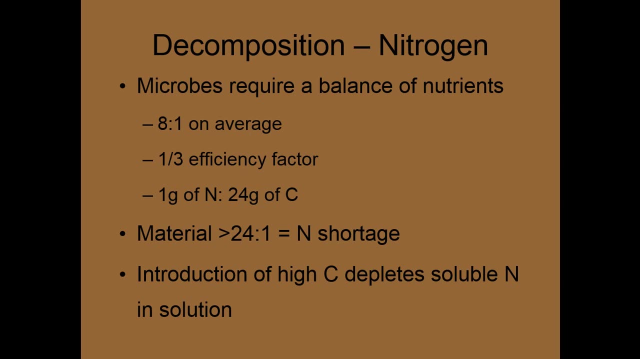 pH and limey requirements, which we spoke about in the previous video. Microbes require a balance of these nutrients, So about 8 carbon for every 1 nitrogen, And so if material is greater than 24, to 1 carbon to nitrogen. 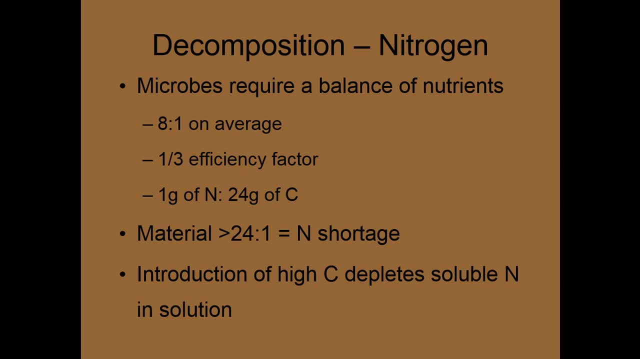 it can cause a nitrogen shortage And when this happens, so the introduction of high carbon depletes soluble nitrogen. So that is where we have an situation where the microbes are using the nitrogen for decomposition and taking it out of solution for the plants. so it's: there's no nitrogen, that is. 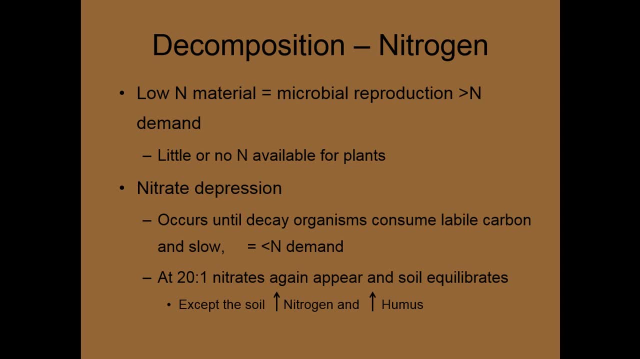 plant available. so this is what we call a nitrate depression of period. so this occurs when decay organisms consume the labile carbon and decrease that carbon to nitrogen ratio until we get down to about a 20 to 1 ratio again, and then nitrates begin to appear and the soil equilibrates high nitrogen materials. so 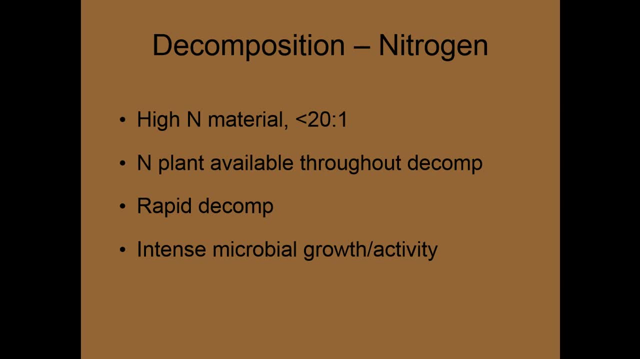 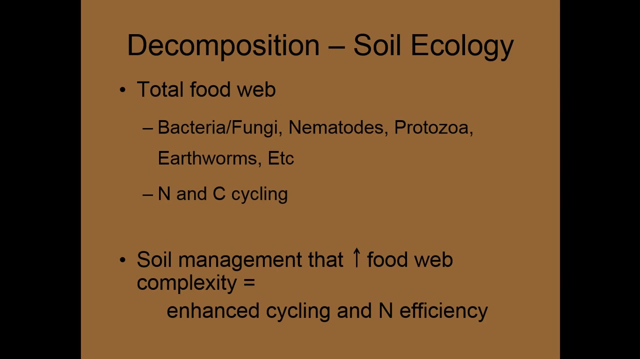 less than 20 carbon per one nitrogen. nitrogen is plant available throughout the decomposition process. that is a rapid decomposition process full of microbial growth and activity, so part of the total food web. looking at total soil ecology, we have bacterial bacteria and fungi, active nematodes, protozoa to earthworms, etc. and nitrogen carbon cycling. so soil